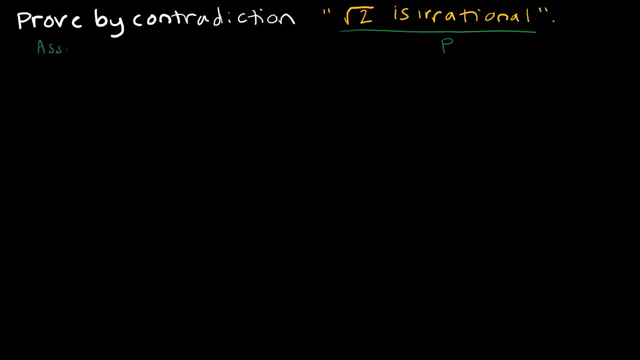 to assume not P. That is how we go about this. So what am I going to assume in this case? I'm going to assume radical two is not irrational, So radical two is rational. Now, a lot of people get to this point, and they 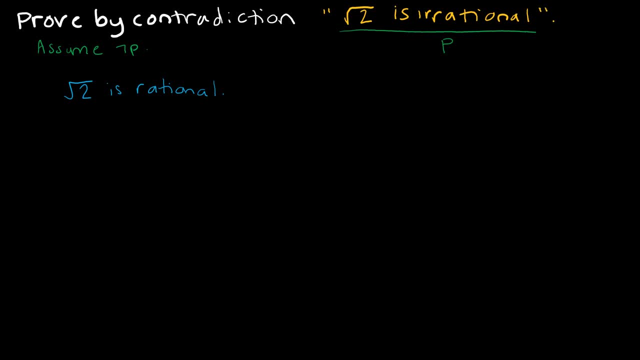 say: well, now I have no idea where to go because I've used everything that was given to me in the question- And you have, except that we are always going to rely on those definitions. So think about what the definition of a rational number is. So I'm going to assume that P is true And I'm going 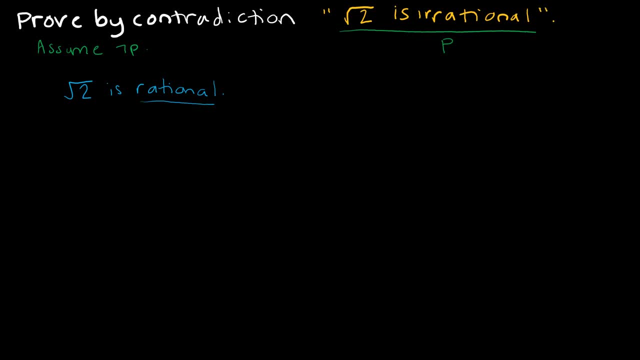 to assume that radical two is rational. So I'm going to assume that P is true And I'm going to use a textbook for that, Feel free to Google that. But based on the fact that radical two is rational, I can say: then there exists two integers and I'm going to call them A and B. 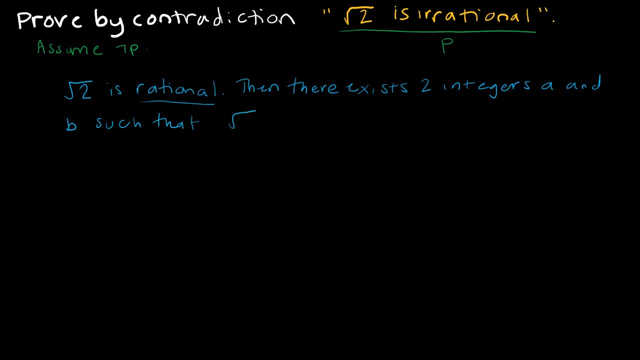 such that radical two can be written as A over B. Again, A is the definition of a radical, B cannot equal zero, still part of the definition. And A and B have no common factors- Again part of the definition, which basically is saying A divided. 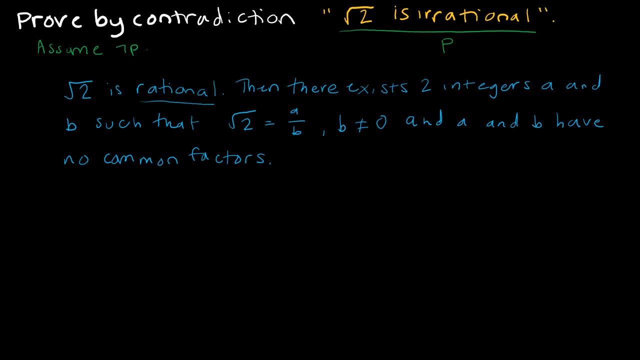 by B. that ratio, which is why it's called a rational number, is in simplest form. So now let's go about the math part of this. So I've assumed that this is true now, Because I'm saying radical two is rational. So I'm going to say radical two is equal to A. 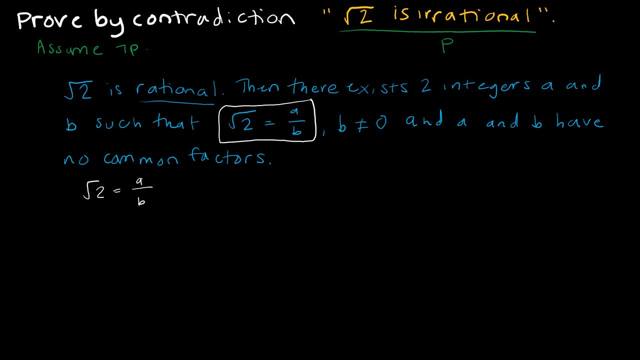 over B. I don't like the radical, so I'm going to square each side. that gives me 2 equals A squared over B squared, And to get rid of the fraction and multiply each side by B squared, So I get 2B. 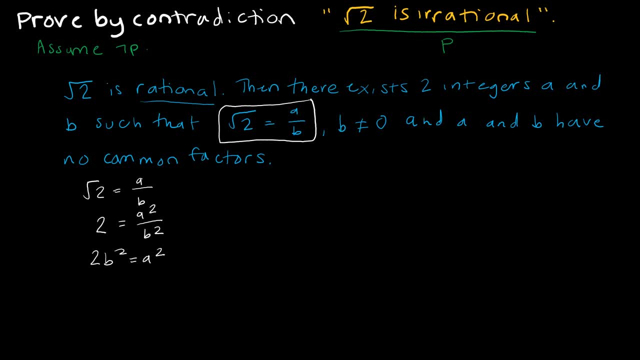 squared equals A squared. What does that tell me? Well, A squared is equal to two times some integer, because, of course, if B is an integer, you will be Amen. Okay. so now let's get together the give and integer, then b squared is an integer. So I can say: therefore, a must be even, And 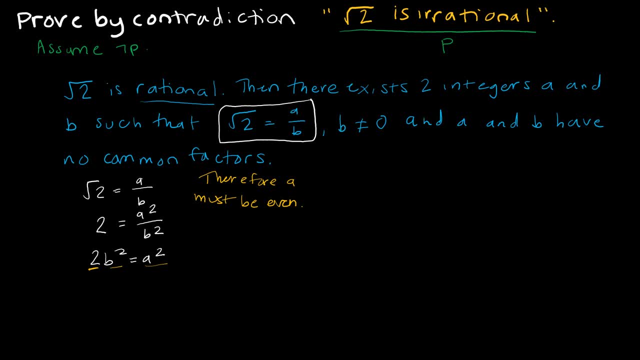 why must a be even? Because a squared was even, and if you square an even number you get an even number. So I'm going to say, therefore, a must be even. So a can be written as 2c, for some c, that is an integer. So now I'm going to take this and continue. I have 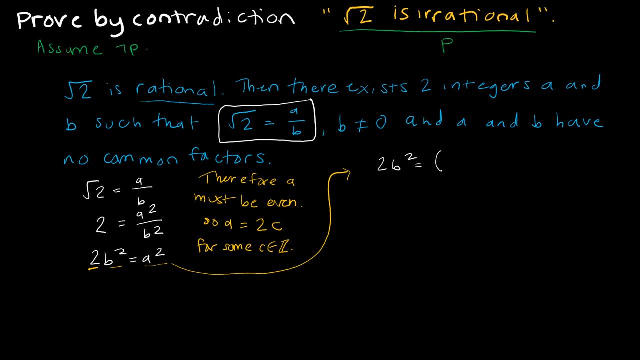 2b squared is equal to a. squared a can be replaced by 2c. 2b squared is equal to 2, squared is 4.. c squared is c squared. Divide each side by 2.. I get: b squared is equal to 2c. 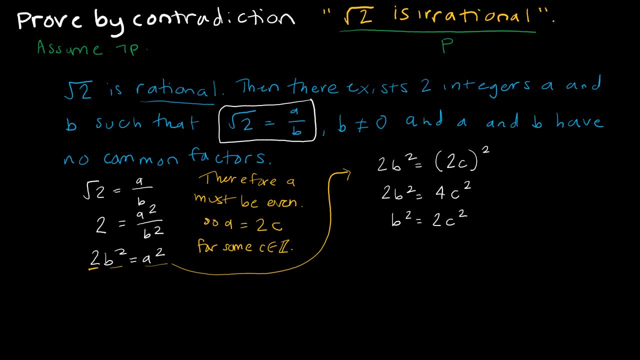 squared And, again, using that same logic, I'm going to say, therefore, b must be even. So why does it matter that I have two even numbers? Well, since a and b are both even, they have a common factor which I said could be even. So I can say, therefore, b must be even, And. 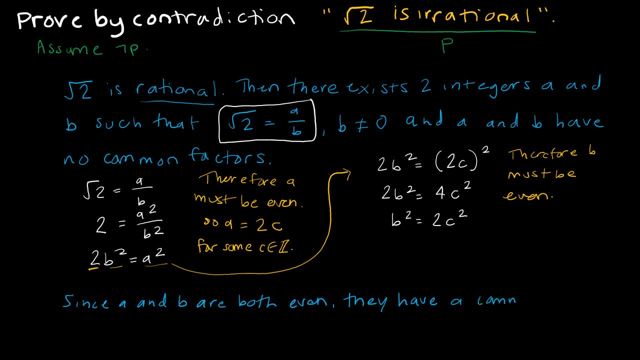 I say another explored And so it does matter that what you said couldn't happen. So they have a common factor. So essentially what I've done is I found a contradiction to what I assumed to be true, that a and b have no common factors. I'm saying, yes, they do. 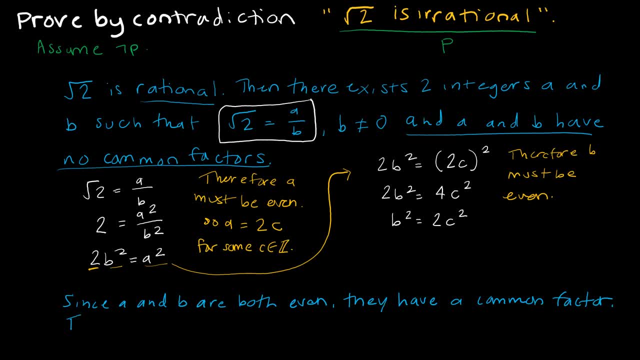 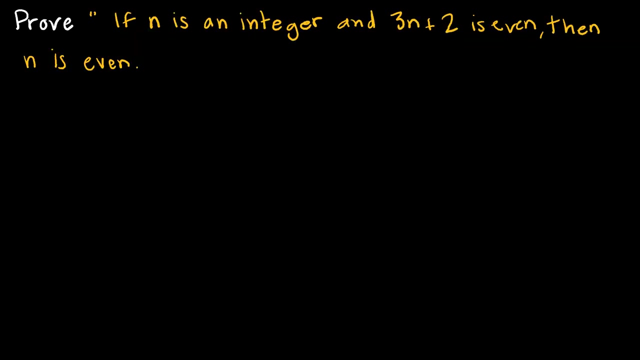 have a common factor. Therefore, radical 2 is irrational. instead, you're correct to call them irrational by contradiction, Or therefore, by contradiction, radical four is irrational or radical two is irrational. So let's take a look at the second type of proof by contradiction, which is when we're 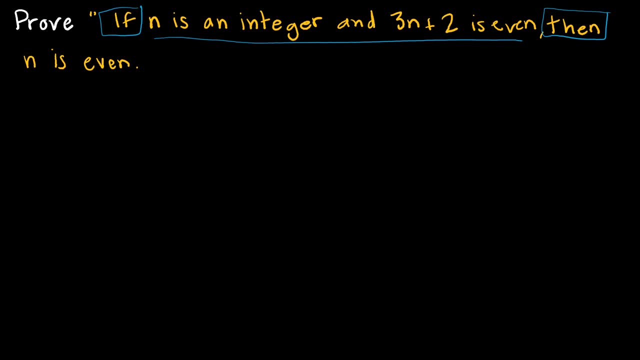 dealing with an implication or an if then statement, And you might be thinking: I think I've proved this already and you would be correct if you joined me for the direct proof video. We've already proved this directly, but let's take a look at how I can prove this now through. 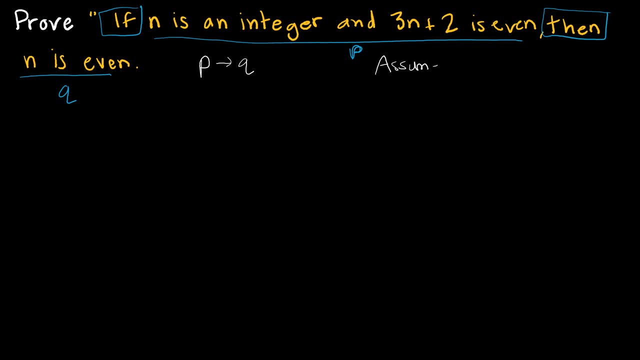 contradiction. Remember, in a proof, by contradiction, of an implication, I'm going to assume P and not Q, and then I'm going to work to either show that if P were true, then Q must have been true, or if not Q were true, then P must have been true. 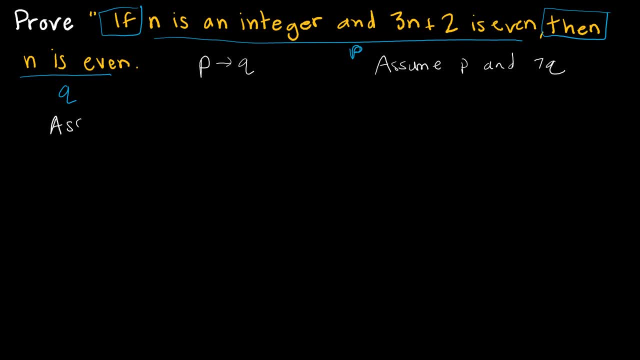 So let's get started. I'm going to assume P, which is 3N plus Q Plus 2, is even for some N. that is an integer And N is not. Q says N is even as Q, so not Q is odd. 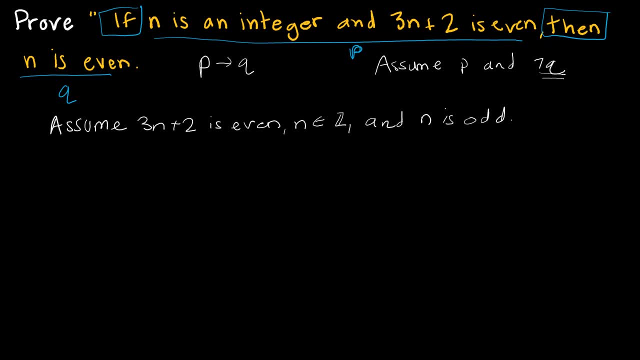 N is odd. So those are my assumptions. going in Again, then you might be thinking: what do I do next? Well, what we do next is we think about what we have and where we're headed. So again, we're trying to show something. 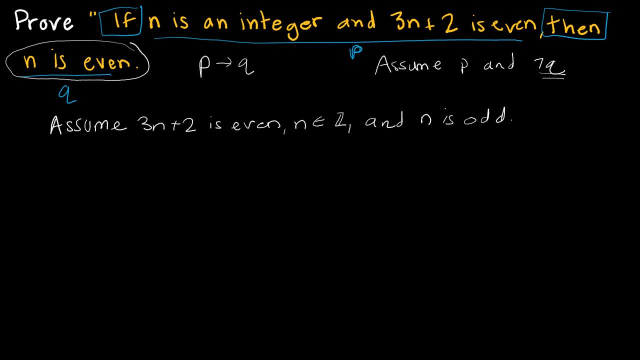 Okay, Something to do with the parity of P and Q, whether or not P is even or odd, Q is even or odd, et cetera. So I'm going to start by saying: since 3N plus 2 is even, then 3N is even by subtraction. 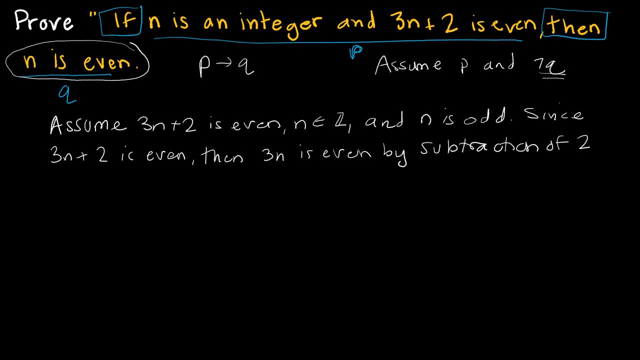 of 2 even integers. Okay, So we know, if we have an even integer and an even integer and we subtract them, we get another even integer or zero, but we're just going to assume even integer. So if I take 3N plus 2 and I subtract 2, then 3N must be even as well. 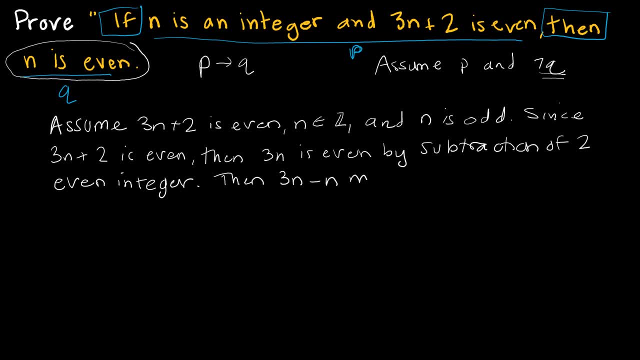 Then 3N minus N must be odd. Okay, So if I take 3N plus 2 and I subtract 2, then 3N is even by subtraction of an even and odd integer. However, if we think about what we just said, 3N minus N is equal to 2N, and I just said.